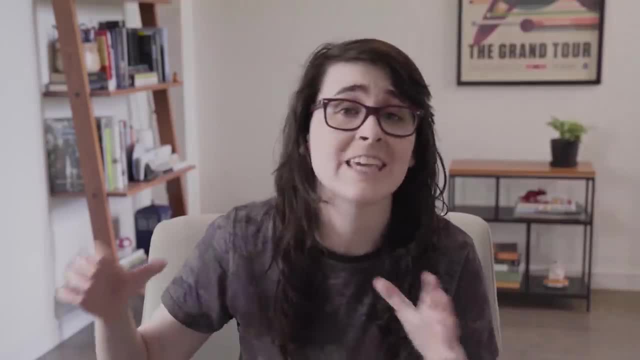 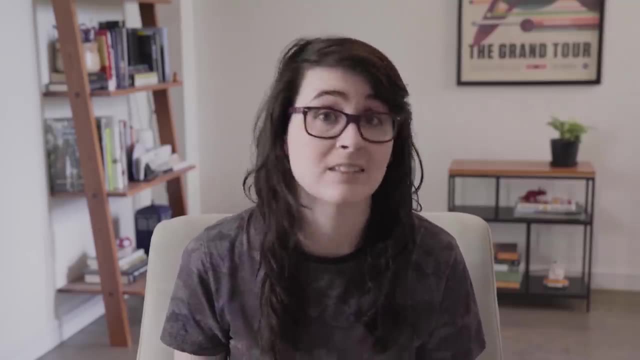 A series on this channel talking about the environment without focusing on the era-defining change happening to our planet right now wouldn't make any sense. Climate change is, after all, the hot mess we all find ourselves in. Climate is the long-term average weather over a particular 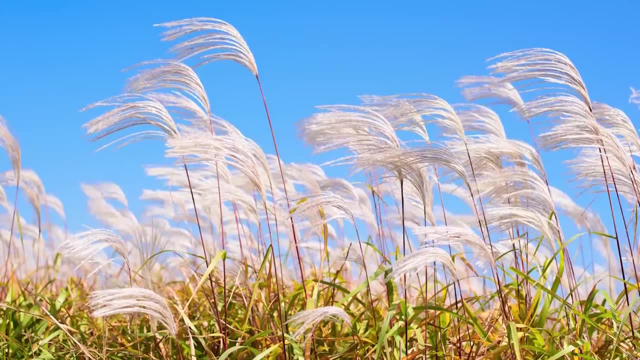 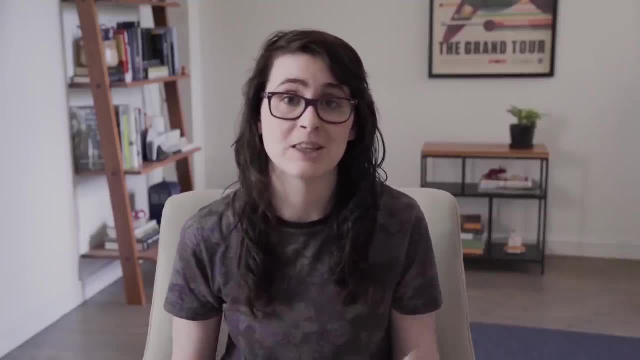 region. It's the typical patterns of temperature, precipitation, wind and how those change seasonally throughout the year. But what does that actually mean? Let's take a trip to a few biomes and compare what climate looks like around the world. We're going to the tropical rainforest. 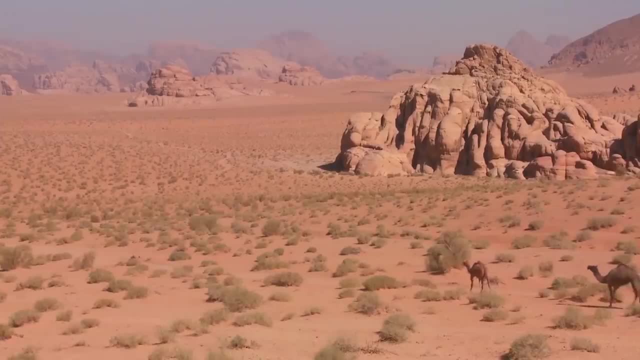 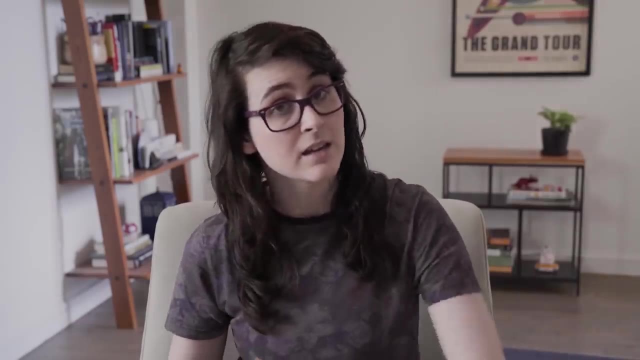 of Brazil, the savannah of Mozambique, the desert in Saudi Arabia and the tundra of Canada. Now, the daily weather might change a lot in these biomes, Depending on the day. the Canadian tundra could be hotter than the desert, But what we're interested in is the 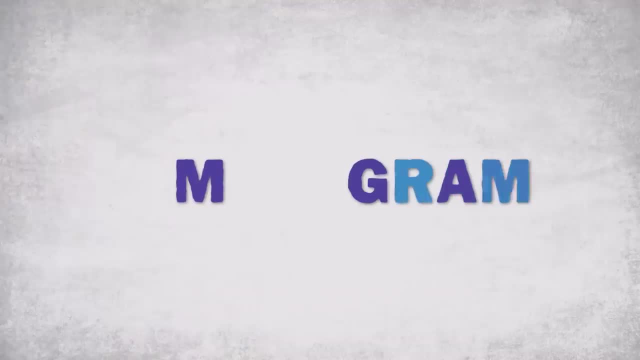 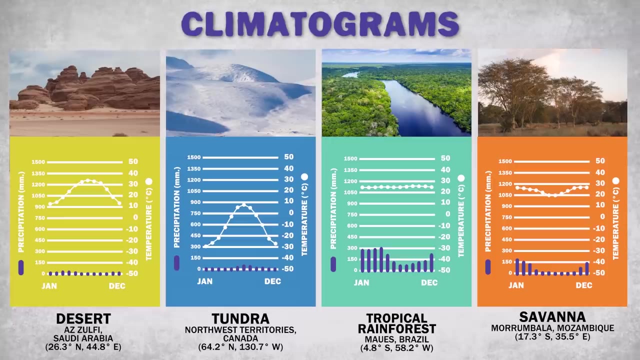 climate. A useful tool for comparing climates like these are climatograms, which visually represent the climate of a region throughout time. This gives us not only an idea of what the climate is- how much rain and how warm- but also the seasonal patterns, On average, the desert and the tundra. 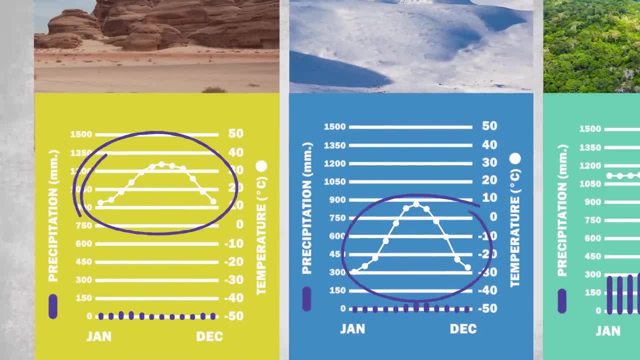 are both very different. The climate of a region is very different from the climate of a region. It's very dry, without much rainfall, but a desert is hotter than the tundra. Tropical rainforests and savannahs are both hot, but you'll see a lot more precipitation in the Brazilian rainforest. 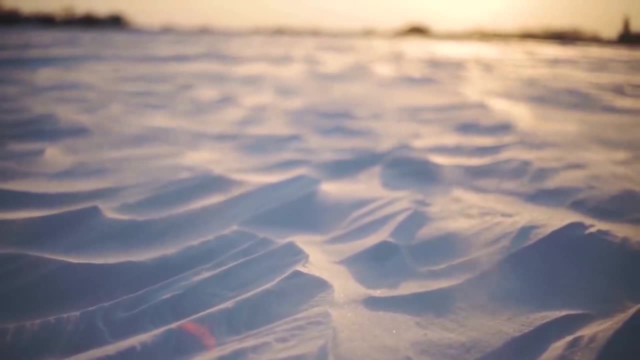 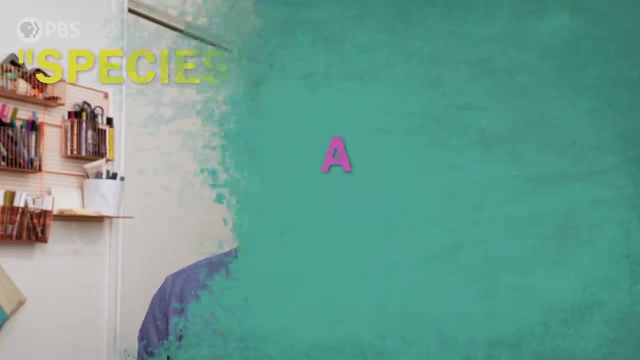 than this savannah. Clearly, climates vary widely from the frigid, dry tundra to the hot and humid rainforest. But what causes all these different regional climates? As Joe mentioned in the first episode of this series, terrestrial biomes are defined by their temperature and precipitation. 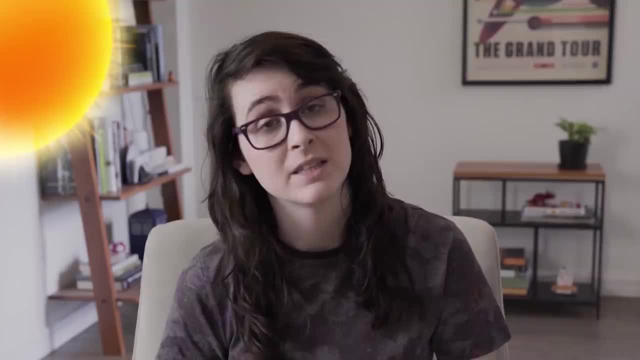 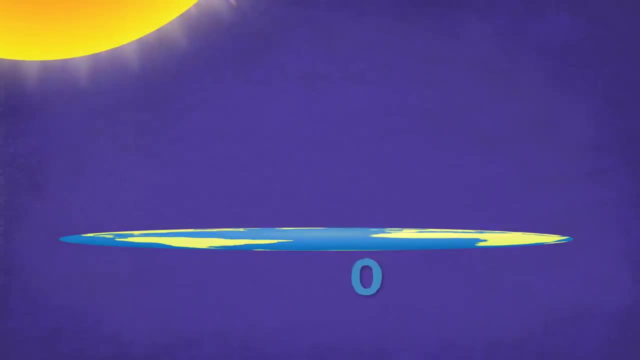 Basically their climate, And the main driver of temperature on this planet, That'd be the sun. Now, if our planet wasn't more or less spherical and was like a flat sheet, everywhere on Earth would experience the same solar insulation. Solar insulation is the amount. 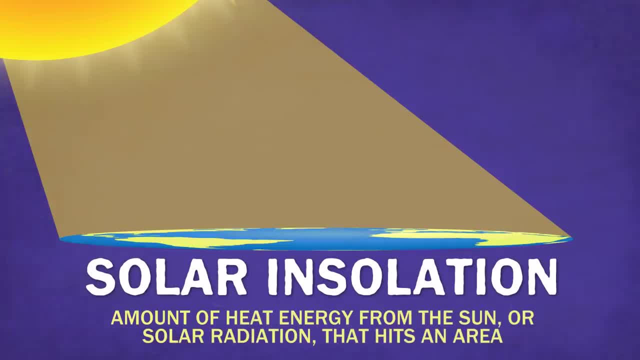 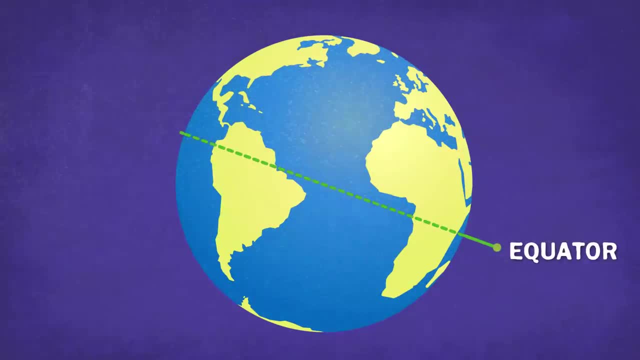 of heat energy from the sun or solar radiation that hits an area, But because Earth is a sphere, solar energy from the sun hits different parts of the globe at different angles. The equator is so warm because incoming solar radiation is perpendicular to the surface Up at the poles. 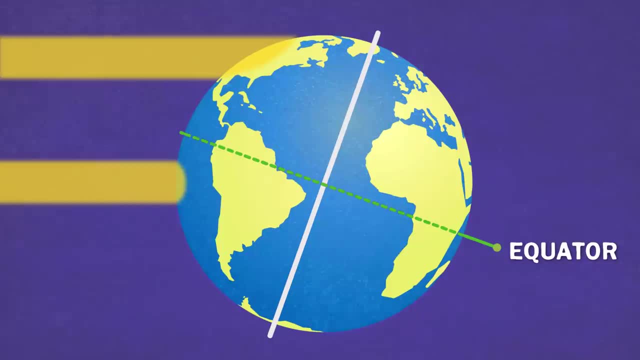 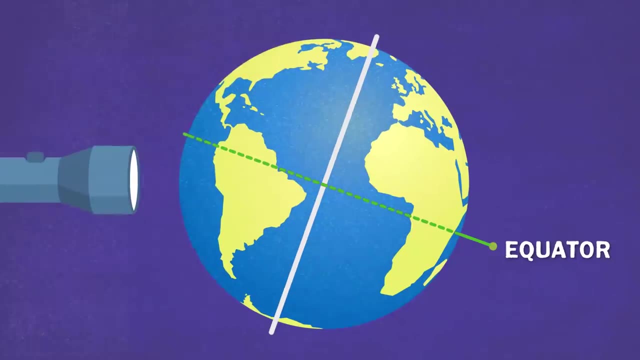 that angle is more oblique, The sun is emitting the same amount of heat energy, but at the equator that energy is more concentrated, while at the poles it's more spread out. Imagine shining a flashlight on a basketball Near the middle. the light from the flashlight is a perfect circle. 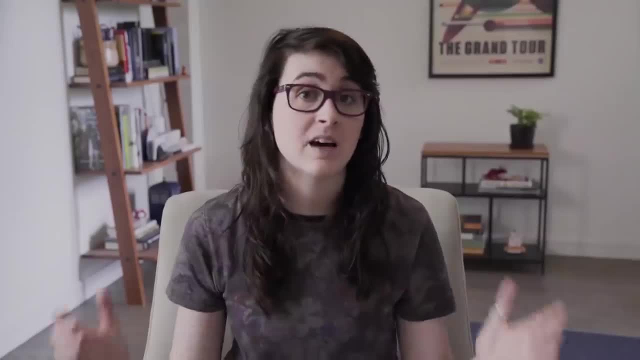 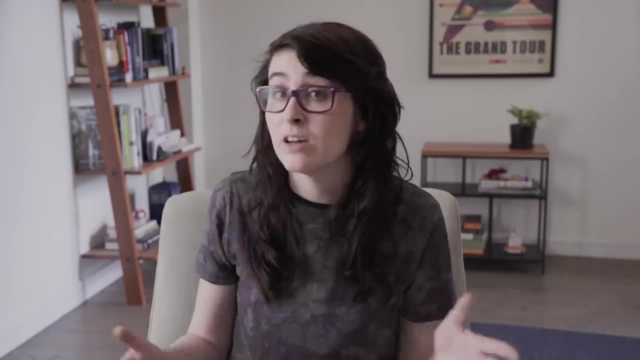 but as you move the flashlight up it becomes more oblong. This unequal heating of the Earth's surface causes the difference in temperature, but it also drives much of the global climate, because sunlight doesn't just heat the ground, it also heats the air. When heated, the molecules of air expand, becoming less dense, and rise As those molecules. 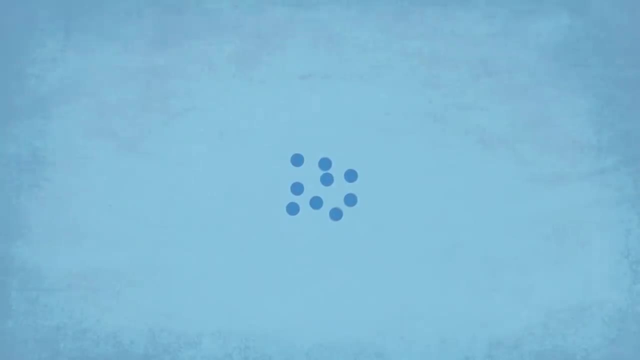 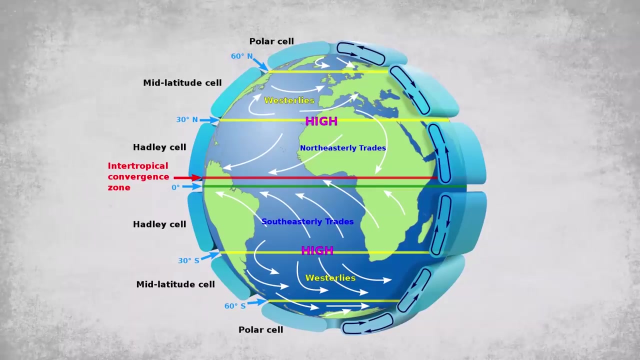 get higher up in the atmosphere, they begin to cool down, become denser again and sink. These rising and falling air masses create global wind patterns that act like enormous conveyor belts: heat, but also moisture. all over the planet. Warm air holds more water vapor. 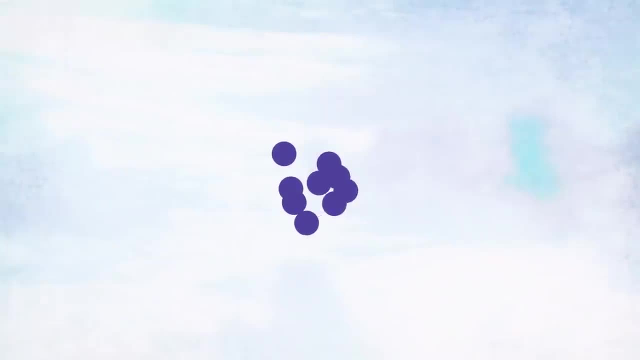 and cooler air holds less. This is because warm air molecules have more energy and move around more, so the water vapor can't condense out. As that air rises, cools and becomes less energized, suddenly the colliding water molecules can condense instead of bouncing off each other. 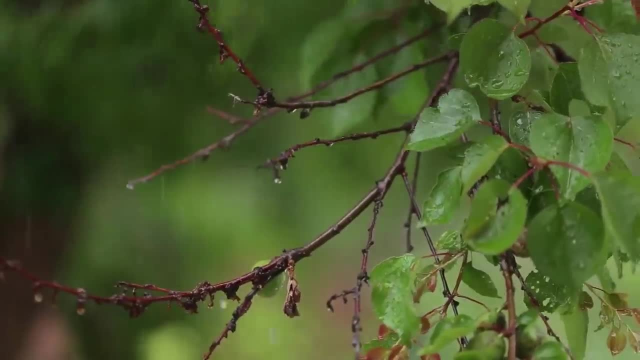 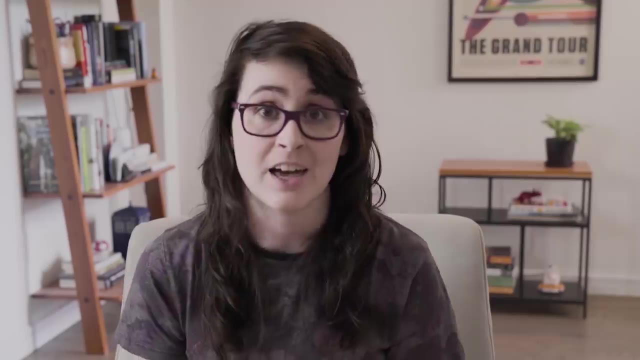 changing from water vapor into liquid water droplets, And that often means precipitation like rain or snow. The heat energy from the sun, spread unevenly across the planet, drives wind patterns and the hydrologic cycle And all together these cycles of wind, rain and heat form. 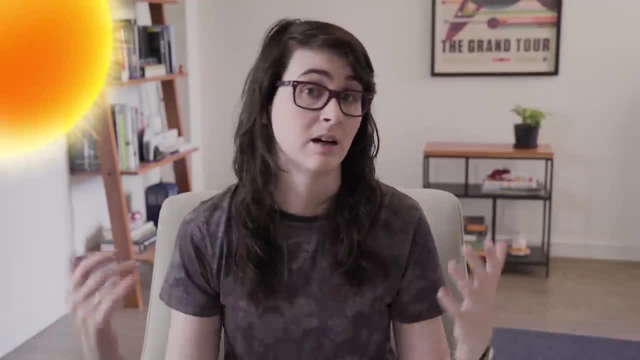 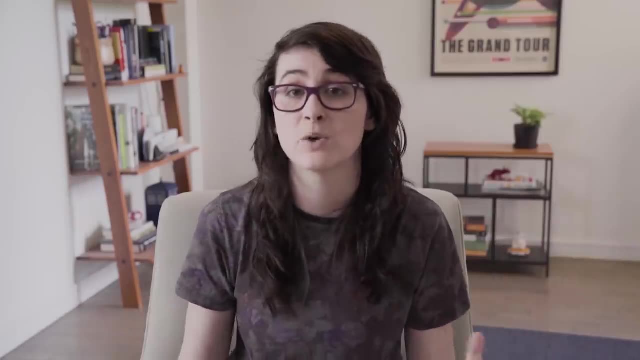 the basis of the variety of climate patterns on earth. The sun and unequal solar insulation on the surface drives the entire climate system. But the sun alone doesn't make all of this work. The earth also has a kind of blanket of molecules that trap some of the sun's heat, and without it, 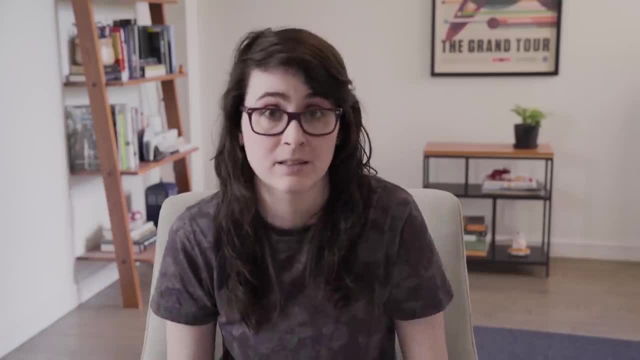 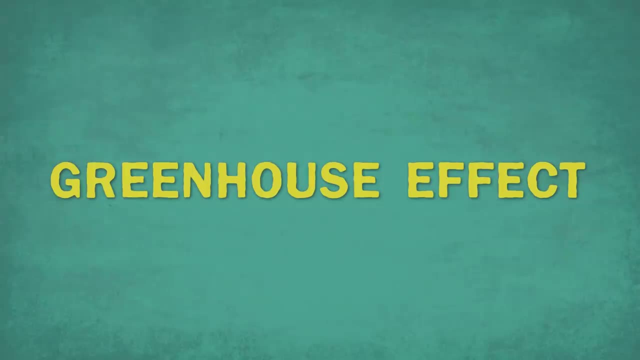 all that solar insulation would hit the earth and then head right back into space. This blanket is the greenhouse effect, and it's what makes our planet livable. Without it, earth's temperatures would swing widely, more like mars or the moon, with freezing cold nights and warm to blazing hot days. The greenhouse effect. 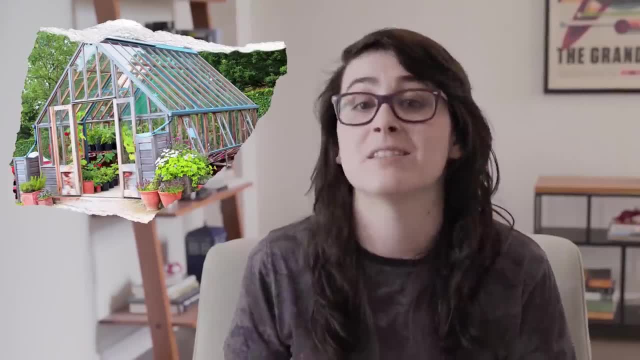 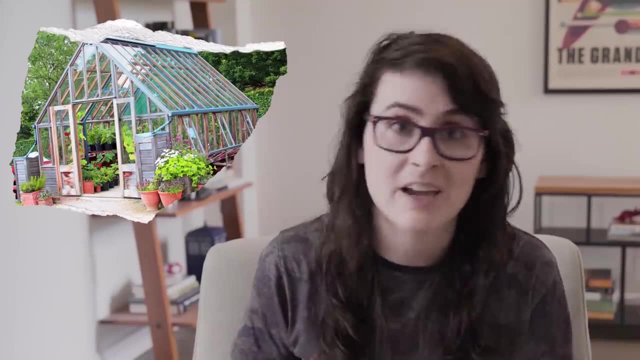 gets its name from well: greenhouses. Greenhouses are great places to grow plants all year long because they trap the sun's heat. The transparent glass or plastic of a greenhouse's roof lets in sunlight, warming the air and the plants and everything inside. 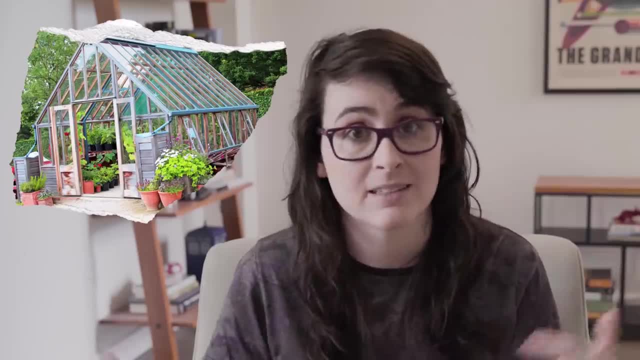 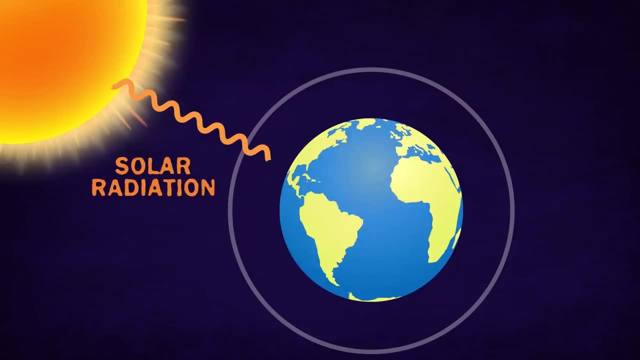 But when that heat energy tries to leave the greenhouse, a lot of it is reflected back inside. The greenhouse gases in the atmosphere do basically the same thing. Incoming solar radiation heat energy from the sun heads toward the earth. A lot of this energy. 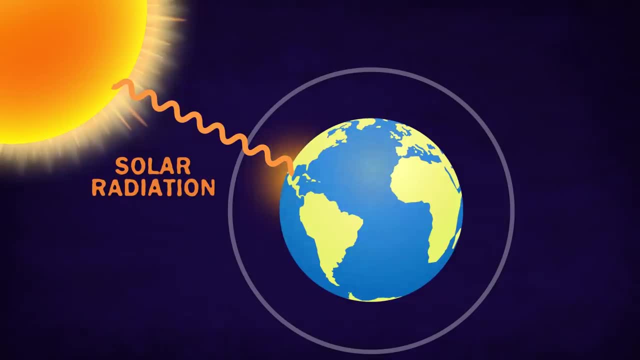 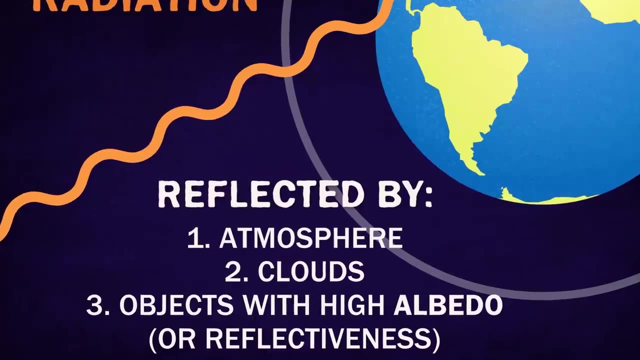 is absorbed by the ground, water trees, warming everything up. Some of it's reflected by the atmosphere and clouds or other objects at the surface with high albedo or reflectiveness, like glaciers, and heads back out into space, Where things really start to warm up and greenhouse. 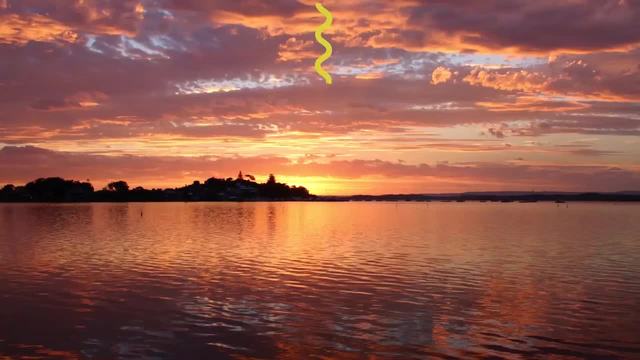 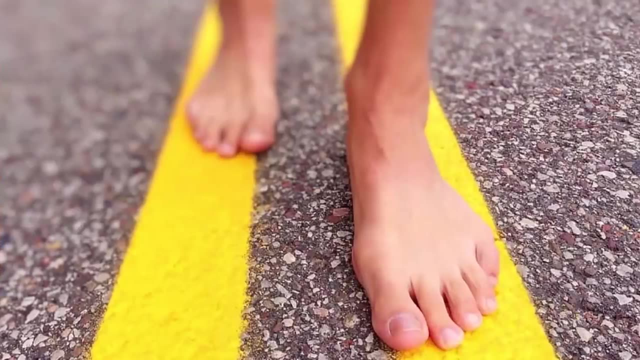 gases get involved is when an object like a road or a lake absorbs all that heat from the sun and it starts to give off heat of its own, which is why walking across pavement without shoes on can be a painful experience in the summer, Compared to the energy from the sun. 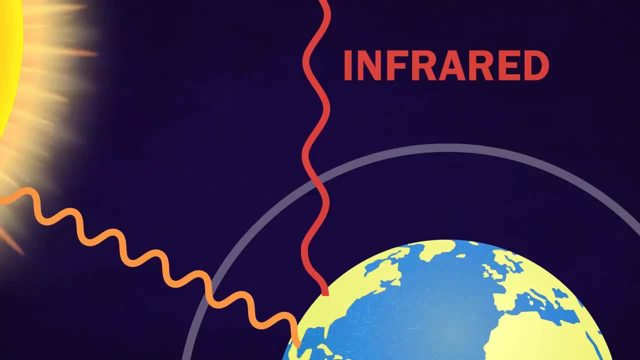 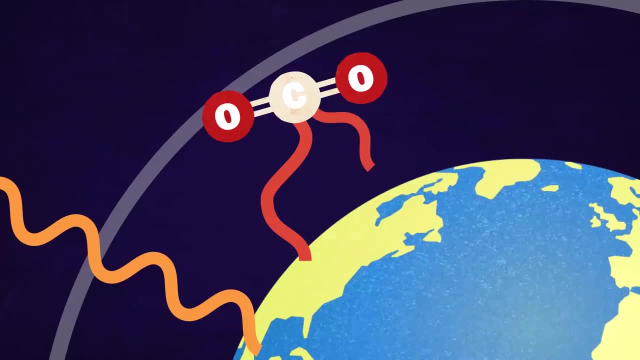 that re-emitted heat has a longer wavelength in the infrared of the light spectrum, and when any of that infrared re-emitted energy hits a greenhouse gas molecule, that molecule is able to absorb that energy and re-radiate it, warming the atmosphere. 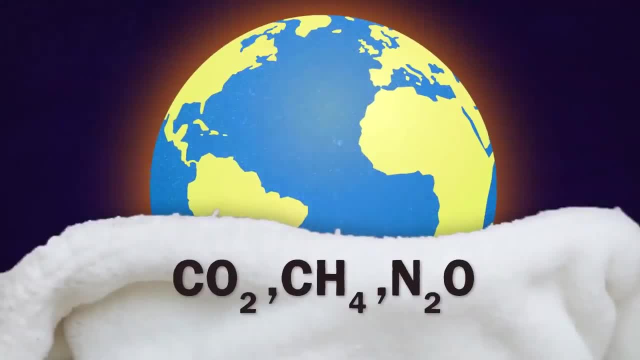 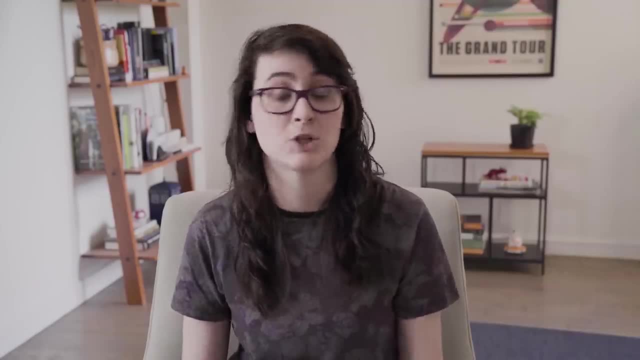 Like a real greenhouse's windows. greenhouse gases are like a big blanket or jacket wrapping the earth, keeping heat trapped inside. The greenhouse gas molecules in the atmosphere play a critical role in regulating the temperature of our planet, keeping things fairly stable without massive temperature shifts between scorching days and frigid nights. But it's a balanced system. Too few greenhouse gases in the atmosphere and things start to get a bit chilly, and when we add additional greenhouse gases we're making the planet warmer. Climate change happens when the balance of greenhouse gases is thrown out of whack. 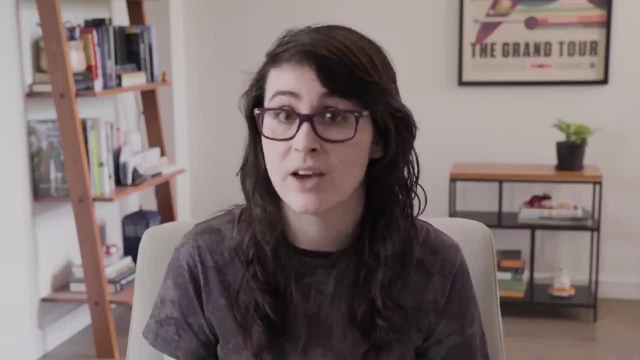 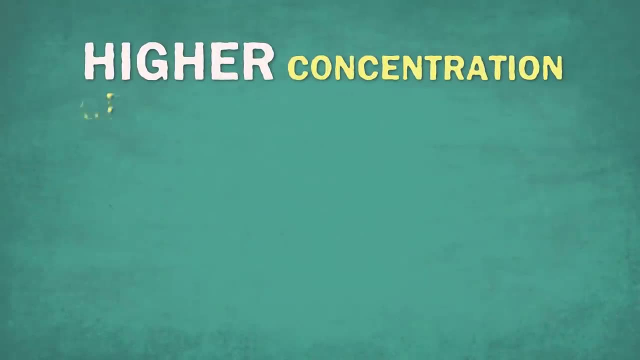 Which means if we and the rest of the organisms on the planet want to live as we do now, then we should be concerned about the amount of greenhouse gases in the atmosphere. Just to make this crystal clear: the higher the concentration of greenhouse gases there are in the 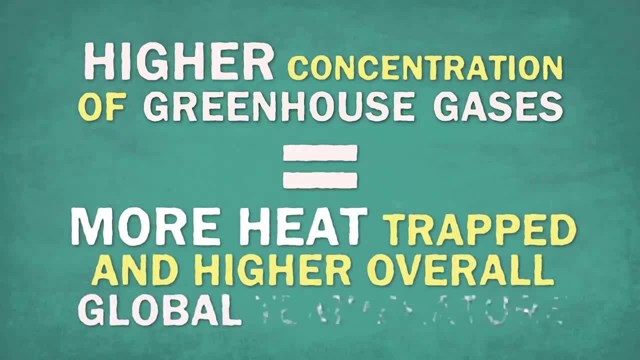 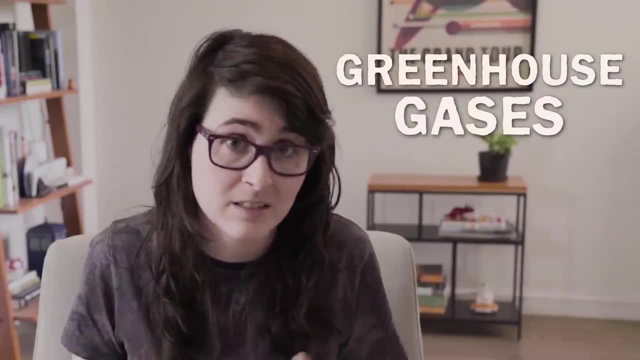 atmosphere, the more heat will be trapped and the greater the overall global temperature. Now that you know what greenhouse gases do, let's talk about what greenhouse gases are. There are a lot of different greenhouse gases because this umbrella term includes any molecule. 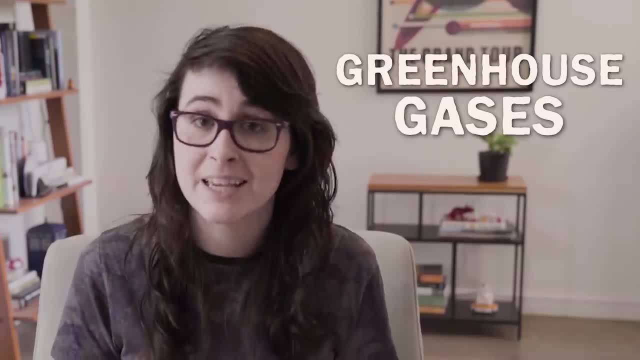 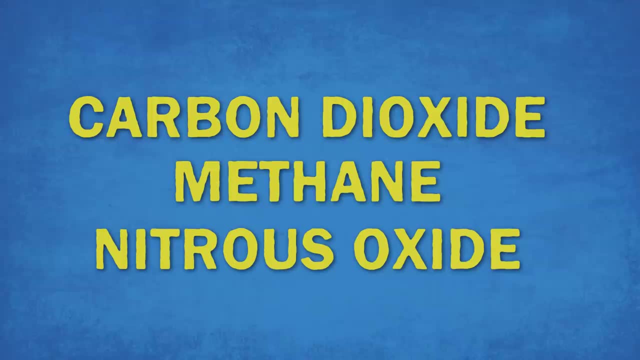 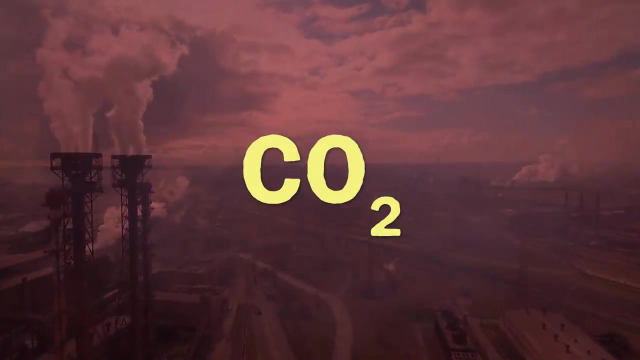 that absorbs outgoing long-term greenhouse gases. So let's talk about what greenhouse gases are. Let's start with carbon dioxide, perhaps the most infamous of the bunch. Let's look at a graph of paleoclimate that reaches way back into geologic history. 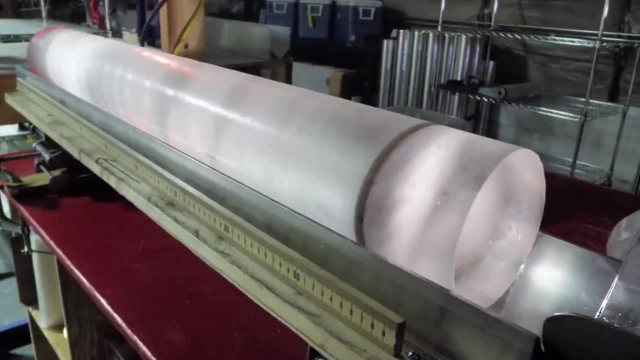 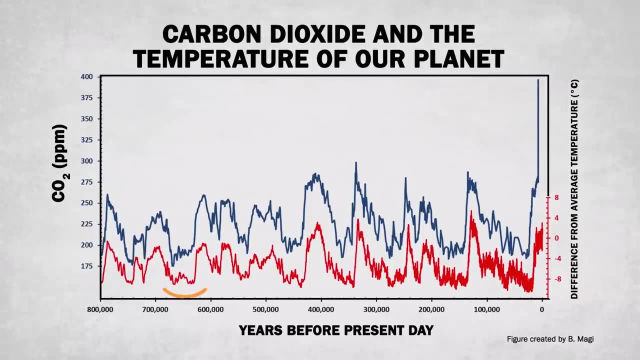 The data behind this chart comes from ice cores, because trapped in long-ago frozen ice are tiny bubbles of air that still look like the atmosphere when they froze. You can probably see a pattern here: When global temperature is low, CO2 in the atmosphere is low. When global temperature is high: 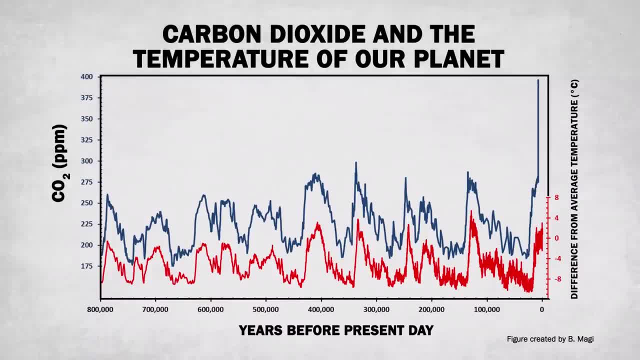 CO2 in the atmosphere is high. Even without doing any analysis of the actual numbers, we can see that temperature and carbon dioxide concentrations are correlated. We can also see that there's a cyclical pattern and that the highs and low points have been. 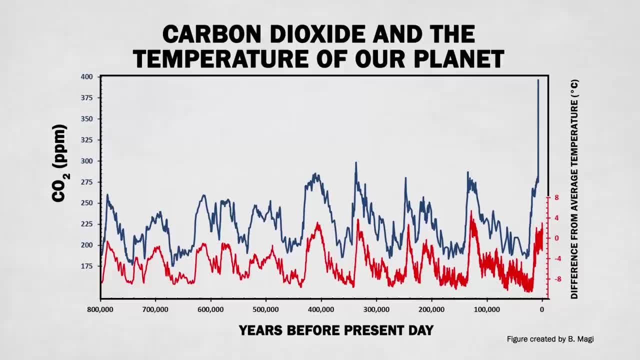 roughly the same as far back as the model goes. These long-term cyclical patterns show the natural temperature and carbon dioxide caused by things like the slowly shifting tilt and orbit of the Earth. And when I say slowly, I mean really slowly. Look at the horizontal x-axis on this chart. 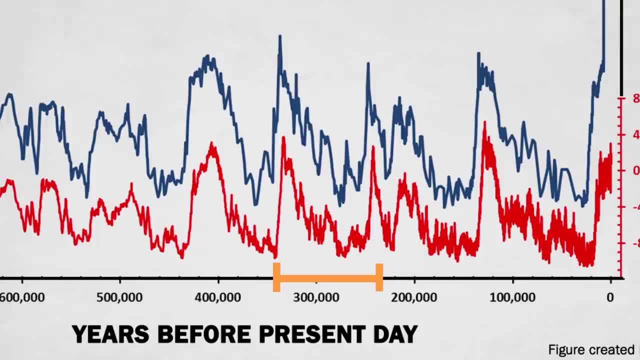 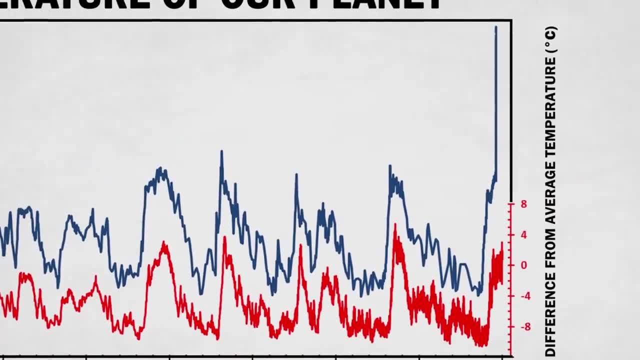 The distance between the peaks is hundreds of thousands of years, a length of time so long that I personally have no frame of reference. for Now, take a look at the end of this graph. Carbon dioxide spikes way up, way higher than we've ever seen in the ice core records. 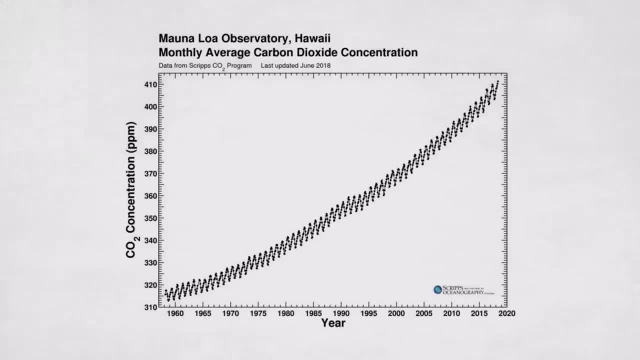 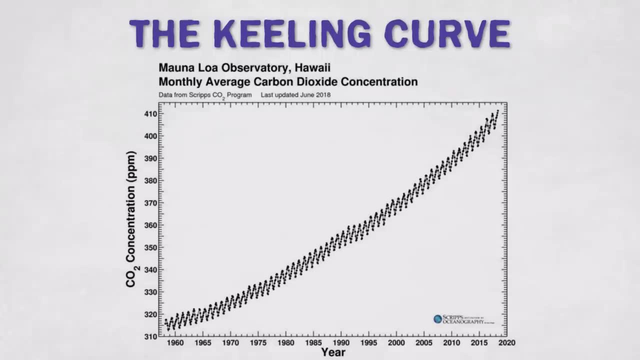 We talked about this chart in the episode on the atmosphere, but this is the Keeling curve, a daily record of carbon dioxide concentrations at Mauna Loa, Hawaii in the United States. There's two distinct trends here: the small yearly fluctuations. 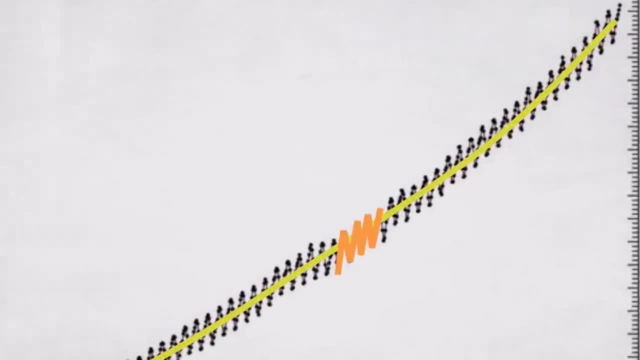 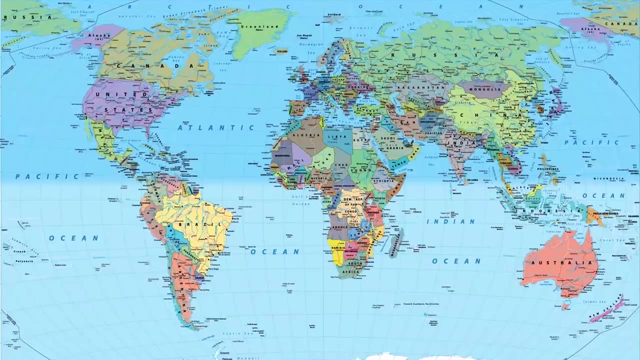 and an overall trend upward. Those yearly fluctuations are because of less photosynthesis and therefore less drawdown of CO2, occurring during the northern hemisphere. winter months, The northern hemisphere has more landmass, so the seasonal cycle of trees and grasses has an impact. 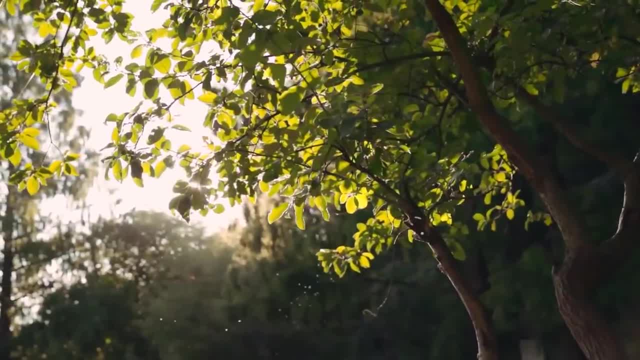 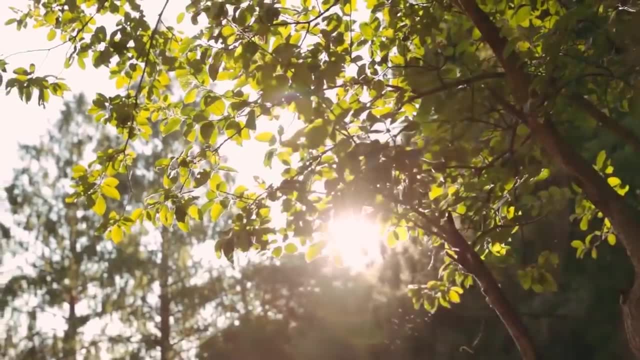 on global carbon dioxide concentrations During the northern hemisphere summer, when all the plants wake up, photosynthesis rates go up. plants draw down carbon dioxide out of the air and transform it into organic compounds. The yearly cycle is natural and expected, and has probably been going on for millennia. It's that upward trend that's worth. 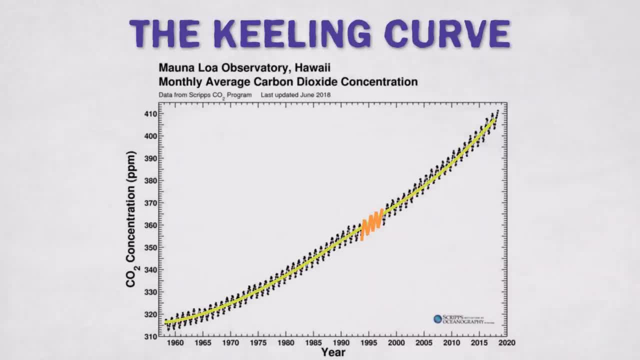 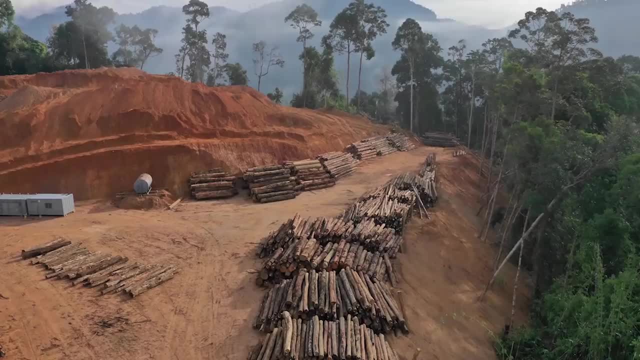 worrying about. And if you look at the numbers, the increase in carbon dioxide concentration is exponential, with the rate of increase growing every year. This exponential increase is because of humans, caused largely by deforestation and by burning fossil fuels for heating, transportation, industrial uses and electricity. 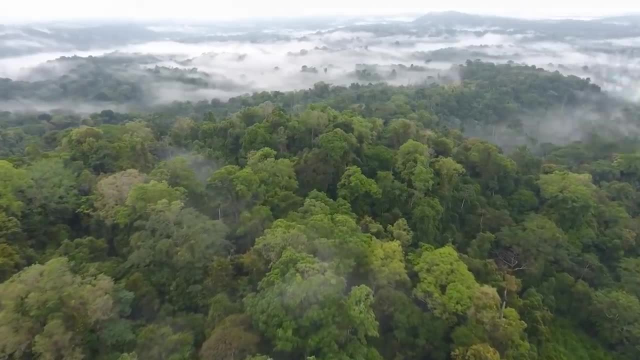 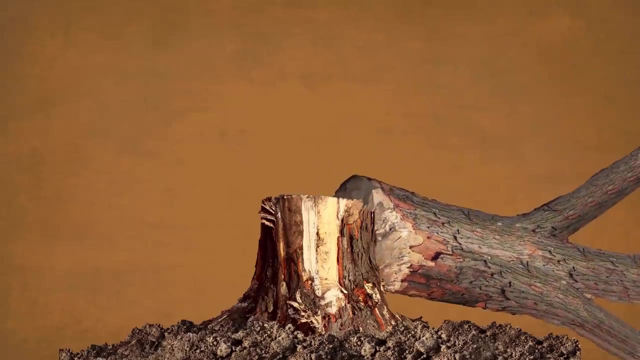 Deforestation is a double whammy, emissions-wise, because forests serve as a carbon sink. Trees sequester carbon in their tissues, trapping it for a long time. Not only does cutting down those trees end up releasing that stored carbon, but it also means fewer old-growth trees to sequester. 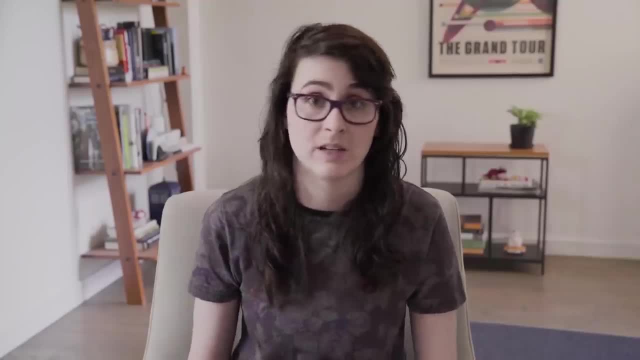 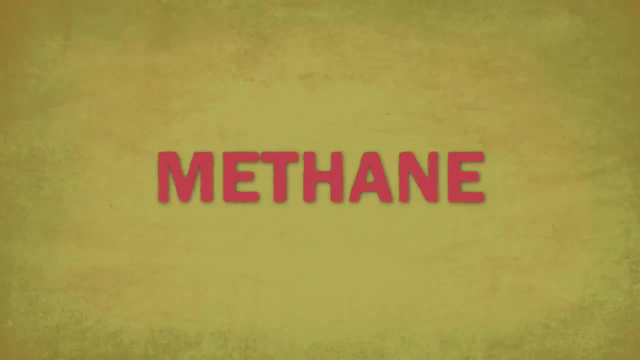 the carbon dioxide in the atmosphere. Reducing fossil fuel use and deforestation is essential to reducing carbon dioxide concentrations in the atmosphere and slowing future warming. Alright, now let's talk about methane. Methane has some naturally occurring sources, like wetlands, but human emissions primarily come from landfills. 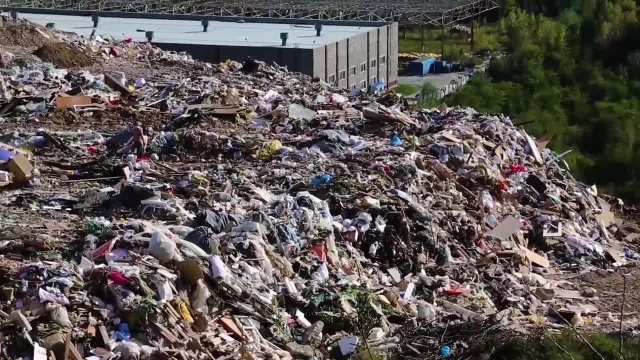 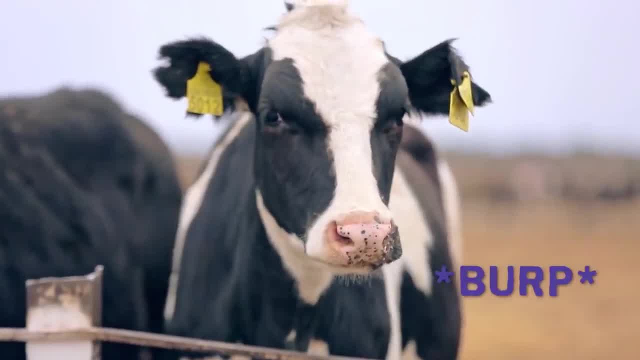 raising cattle and the gas industry At a landfill. the organic material buried inside of all that trash starts to decompose in anaerobic or oxygen-free environments. Cattle produce methane as part of their digestive process And with millions of farmed cattle on Earth, 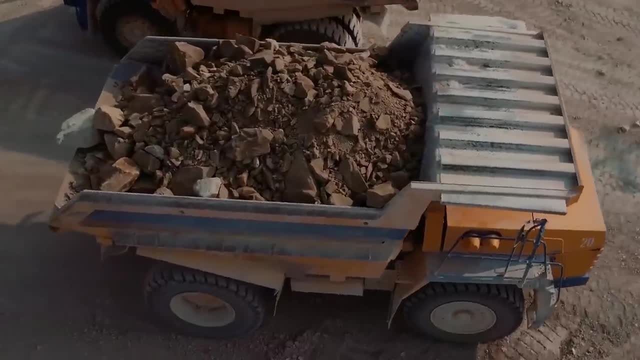 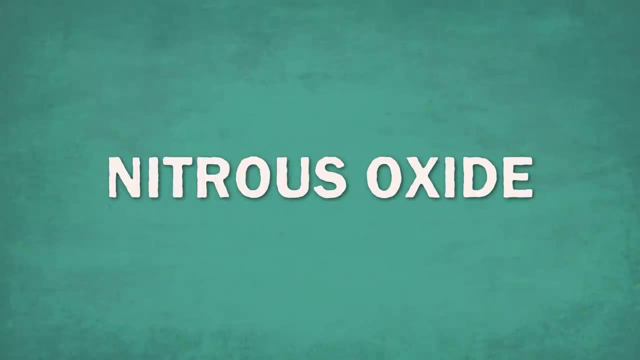 those cow burps make up a major methane source, And mining, transportation and use of the gas, which is mainly methane, are also serious sources. Finally, we have nitrous oxide- Technically laughing gas, but definitely not funny. This greenhouse gas is generated as a byproduct of fertilizer on agricultural fields. 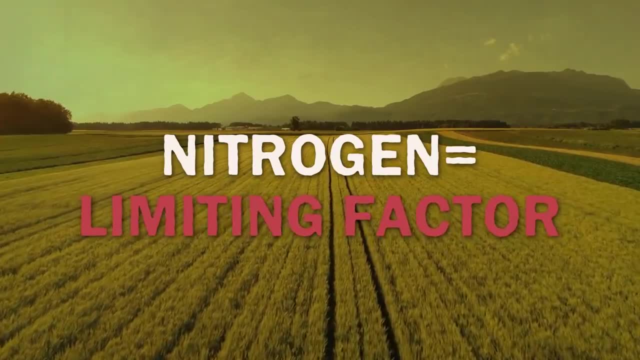 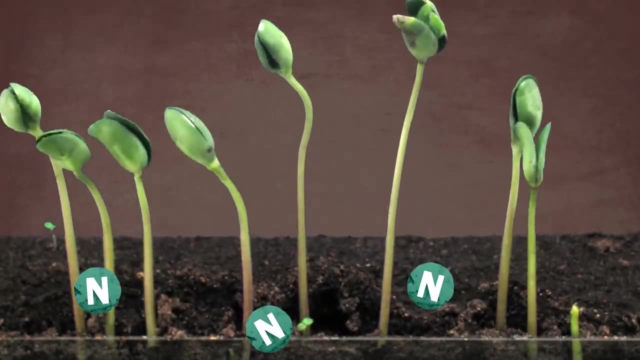 Nitrogen is one of the limiting factors in most soils, regulating how many plants can grow. To increase the yield and to maintain soil fertility, farmers add nitrogen to their fields. While that helps the plants grow, bacteria in those fields convert that nitrogen into nitrous. 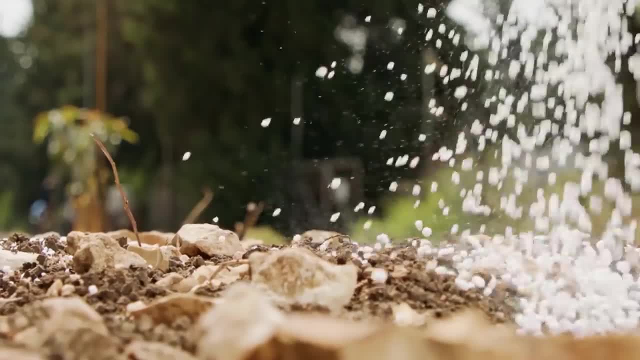 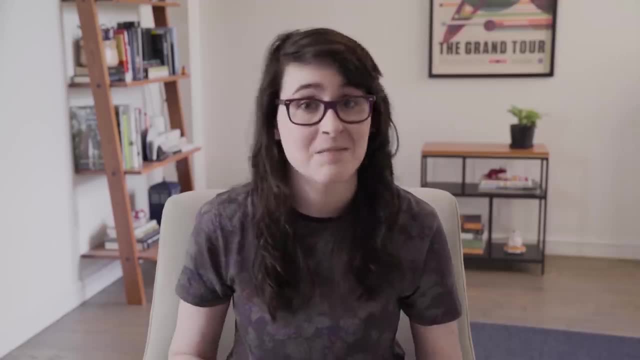 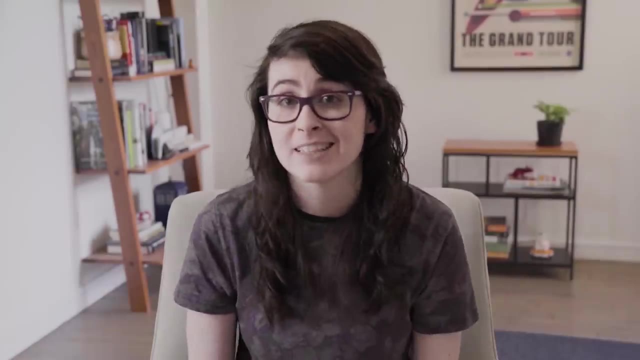 oxide. The more fertilizer used, the more nitrous oxide emissions. Even though it is well understood that increased greenhouse gases cause climate change, emissions of all these greenhouse gases- carbon dioxide, methane and nitrous oxide- are still rising, Which isnot great, But why? What does increased greenhouse 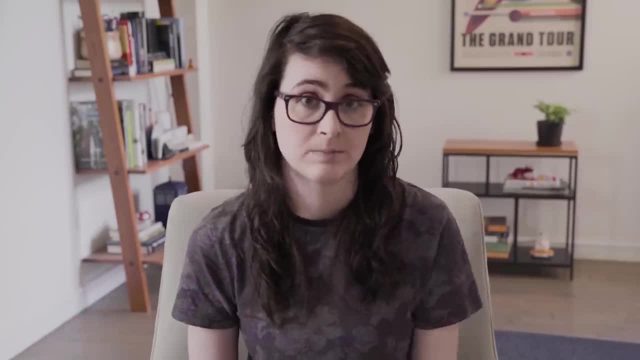 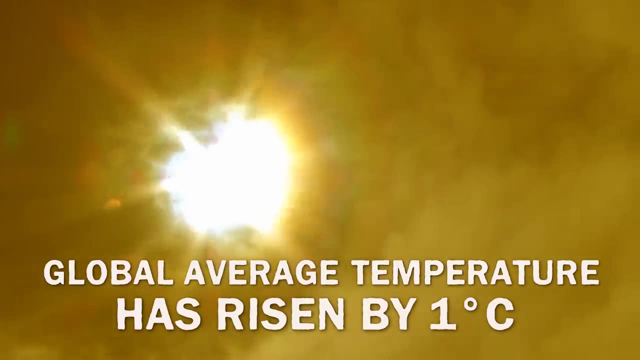 gases and the resulting climate change actually mean for humans and the environment? Well, the obvious: It'll get hotter, And it has. The global average temperature has already increased more than one degree celsius since the 1800s, But that's just the global average. 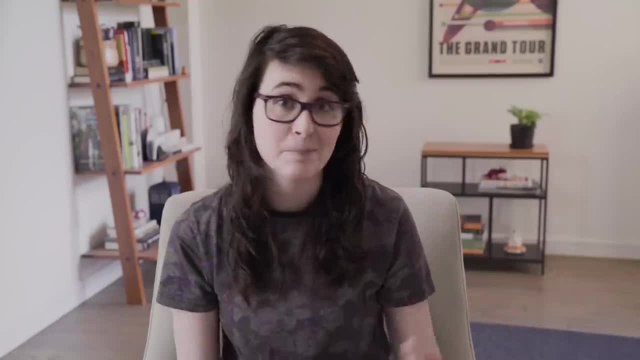 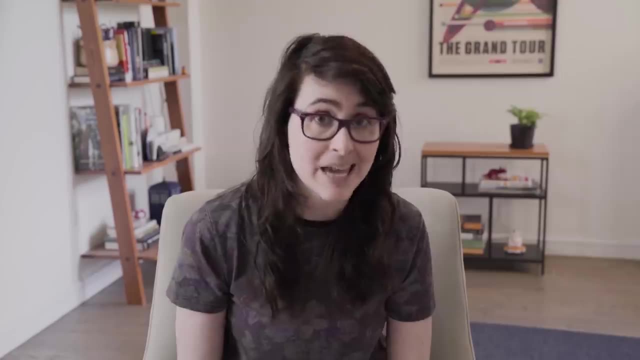 Some places are getting warmer faster, like the poles, And temperature going up alone isn't the only issue, Because the planet warming also causes changes in the climate. At different temperatures, molecules in the air and ocean behave differently, So as things heat up, we see changes in wind patterns, precipitation and ocean currents. In some areas, this means increased droughts and forest fires. In others, more frequent floods and stronger hurricanes. Devastating hazards also aren't the only impact of climate change As parts of the planet. change the climate changes and the climate changes As parts of the planet. 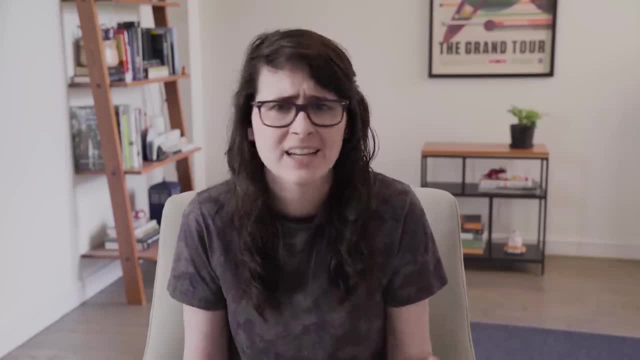 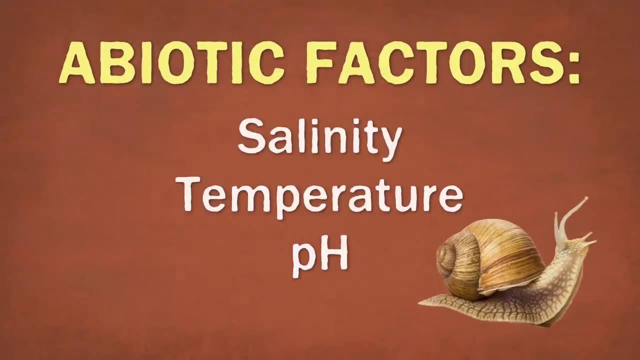 become warmer, we also see habitats disappearing or shifting, with dramatic consequences for the biosphere. Every organism has a range of tolerance for abiotic factors like salinity, pH and temperature. If those factors become too extreme, the organism has to move or die. Some species have 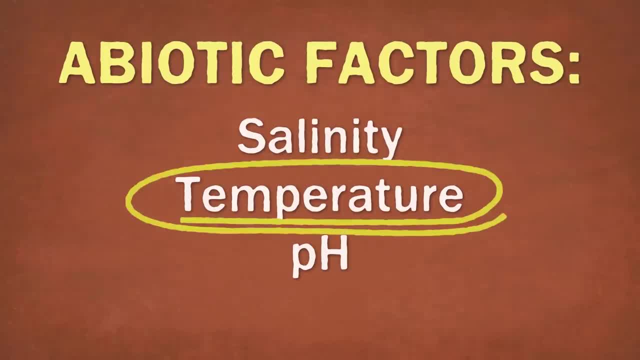 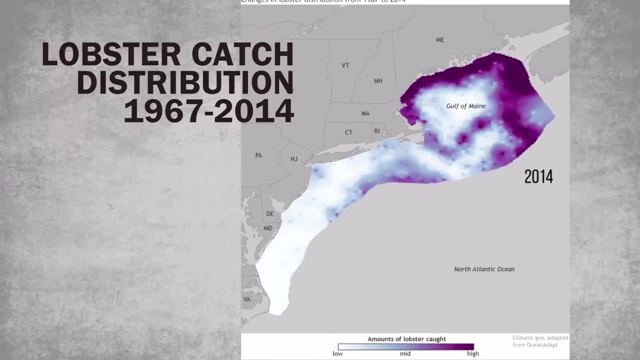 been moving their home ranges in response to changing temperature patterns. For example, lobsters of the eastern coast of North America are shifting northward in search of cooler waters, But other species where moving isn't as easy, like certain tree species, are disappearing. 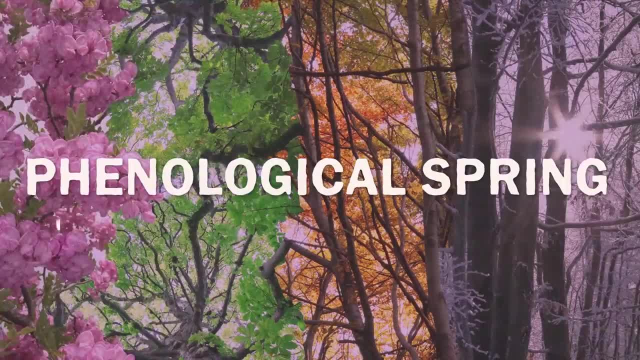 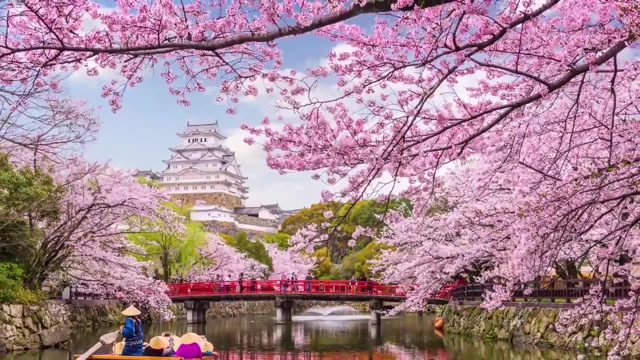 Climate change is also messing with the seasons, Phrenological spring, the time of year when plants start to bud. new growth has occurred earlier, in response to a warming planet. For instance, researchers have tracked the date the cherry trees blossom in Japan, based on centuries of diary entries and chronicles. 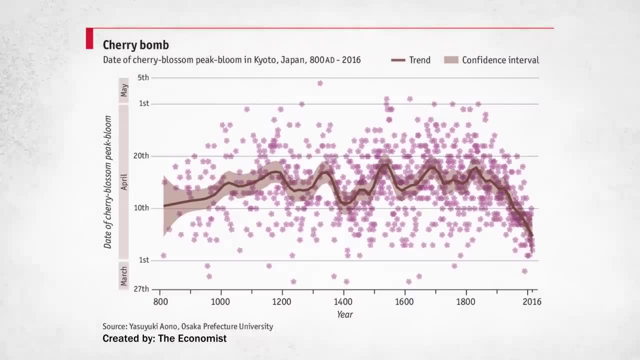 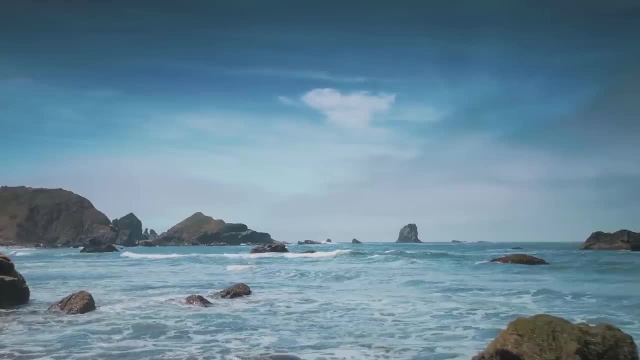 After 1200 years of a nice steady cycle, the peak for cherry blossoms in Japan has been getting earlier and earlier. thanks to climate change. The oceans are becoming warmer too, and, as you may remember from episode 3, the oceans make up a huge portion of the planet, so increased temperatures in the oceans have. 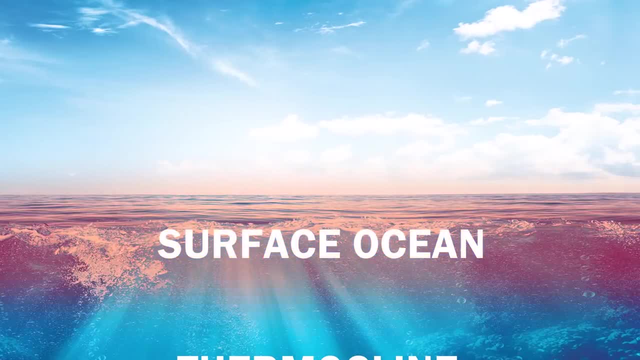 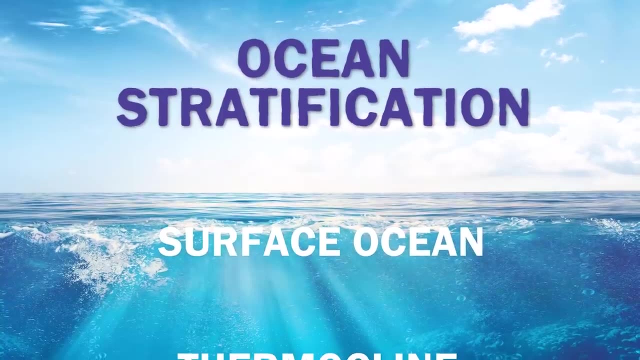 ramifications all over. The oceans are warming fastest at the surface, which leads to an increase in a thing called ocean stratification. Basically, the ocean, or really any mildly deep body of water, has layers with distinct temperature and light infiltration Because the surface water warms. 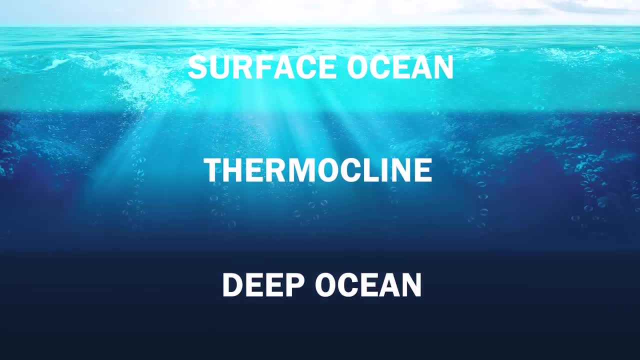 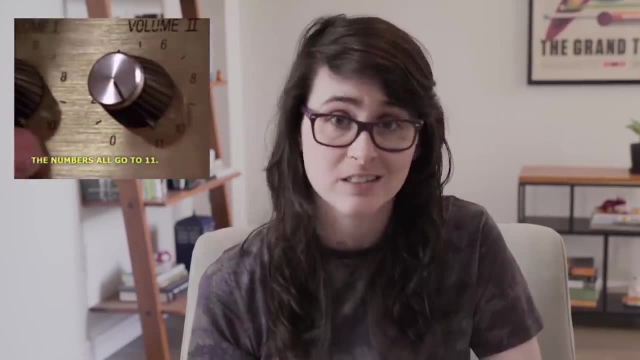 faster than those below. this increases the distinction between the upper layers of the ocean and lower layers. Some stratification is normal and important for nutrient flow but, like most things, when you turn the dial to 11, we start to see problems. 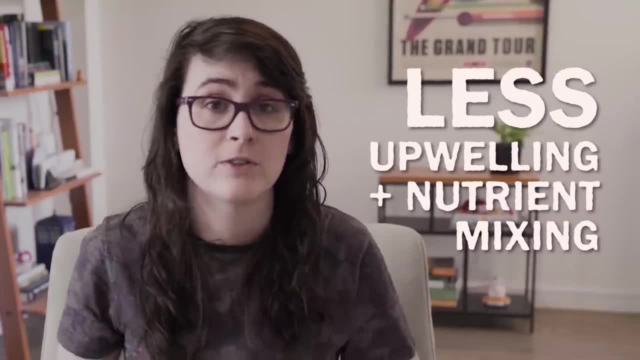 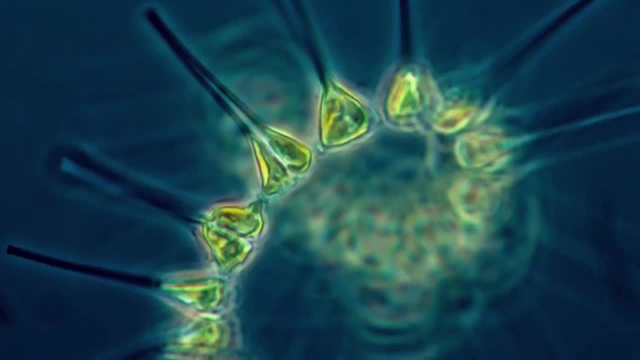 like less upwelling and nutrient mixing, which usually brings cold water full of nutrients to the surface. Without the flow of nutrient-rich deep water, ocean surface organisms can't survive Phytoplankton, a broad category of microalgae that likes to float around the surface. 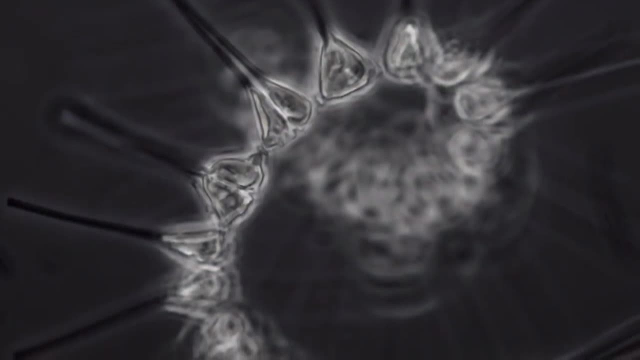 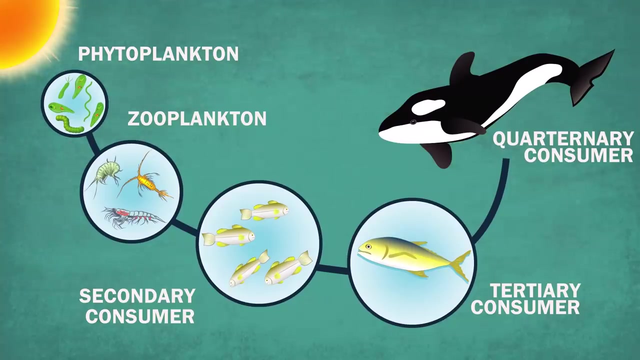 don't do super well without those nutrients, Which would be bad on its own, because phytoplankton are an integral part of the marine food web, acting like terrestrial plants converting energy from sunlight into their little bodies, But plankton are, through the sheer amount of photosynthesis. they do both a major source of oxygen and pull literal tons of carbon dioxide out of the atmosphere, Both things we humans rely on for a stable climate. Increasing ocean temperatures also means rising sea levels, Like the air. as water temperature increases, the energized water molecules take up more volume. 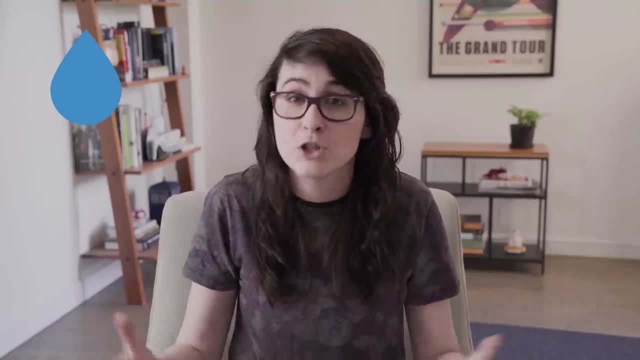 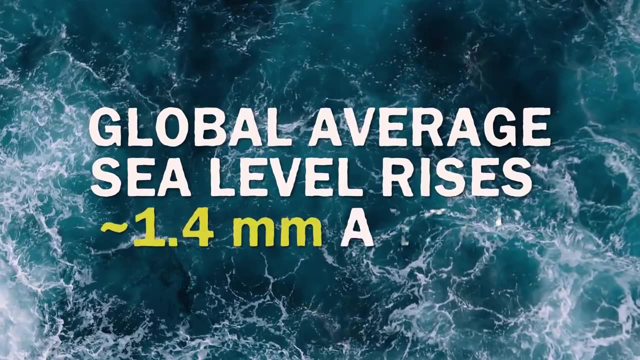 One drop of water expanding a tiny, tiny bit doesn't change much. but when you multiply that by the immense volume of an ocean, from this thermal expansion alone, global average sea level rises 1.4-ish millimeters a year, And increasing temperatures also melt ice. Ice melt from. 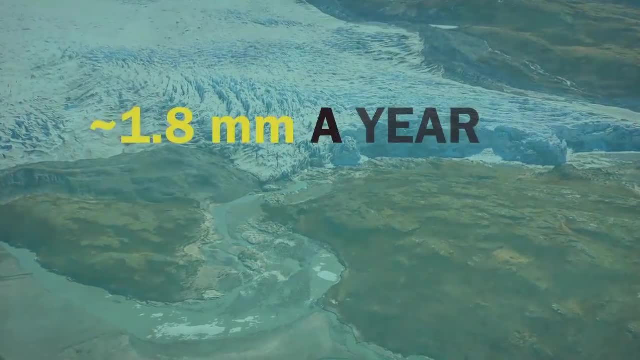 land-based ice, like the Greenland Ice Sheet, accounts for 1.8 millimeters a year of global average sea level rise. Increasing ocean temperatures also means rising sea levels. A few millimeters is admittedly very small if you're thinking about your local beach, but this is 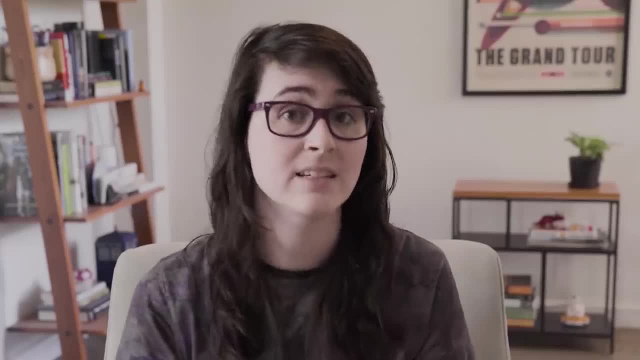 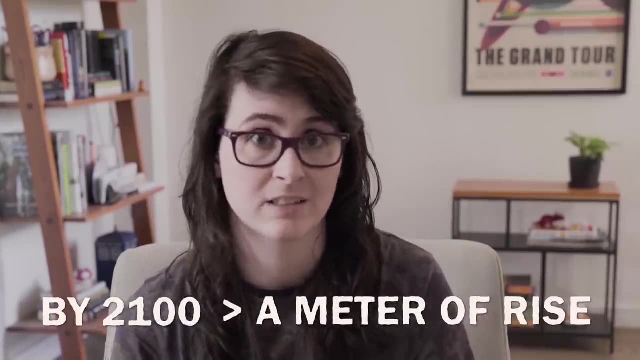 average rise. so in some places ocean levels are rising faster And it's rising a few millimeters every single year And that adds up, This means by 2100 we could see more than a meter of sea level rise, Which again might not sound like much, but when you consider the risks of storm, 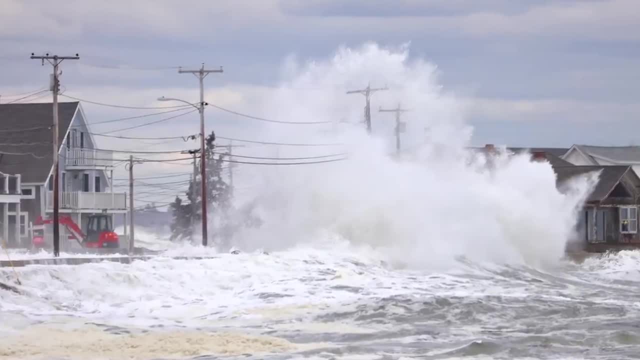 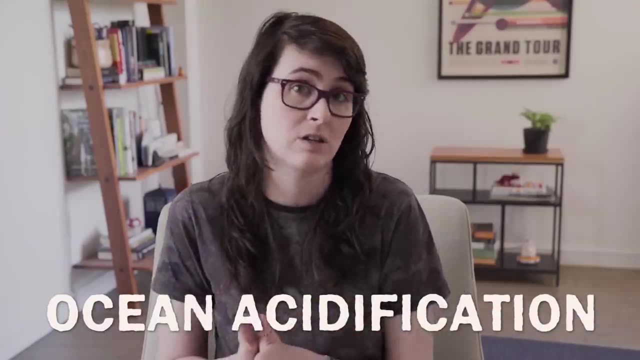 surge and coastal flooding. every extra centimeter puts coastal communities and millions of people at risk. Pumping carbon dioxide in the atmosphere doesn't just raise ocean temperatures, it also causes ocean acidification. But all that extra CO2 in the ocean turns into carbonic acid and drops the pH of the water, taking a normal part of the 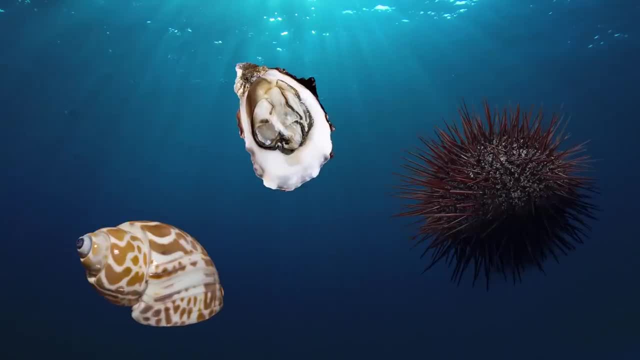 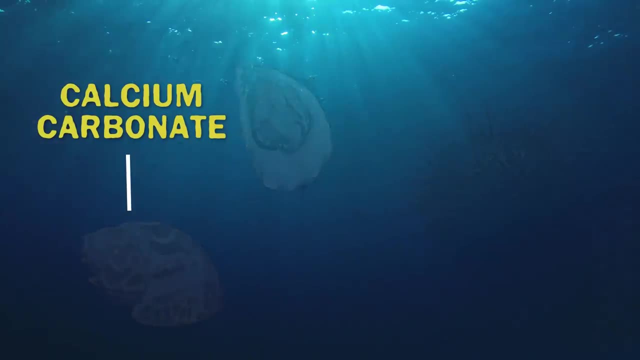 carbon cycle and supercharging it. Shellfish and other organisms that construct their cells and skeletons out of calcium carbonate are literally dissolving away or having a hard time growing their shells in the first place because of ocean acidification. Of course, all the impacts of 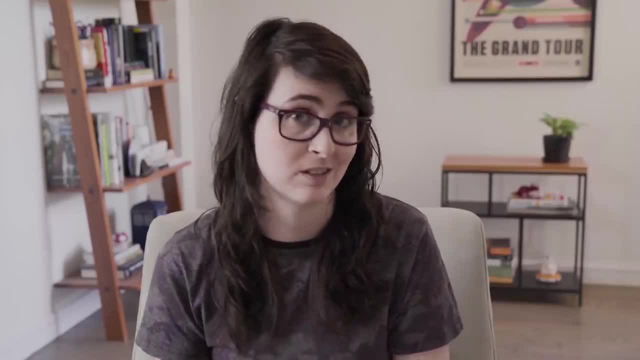 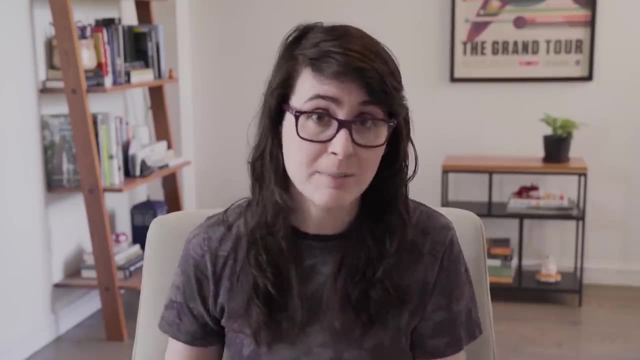 climate change on the biosphere affect humans because we rely on their ecosystem services. As we've talked about in previous episodes, the oceans, atmospheres and soil provide the backbone of the entirety of human society. When climate change starts messing up those systems, 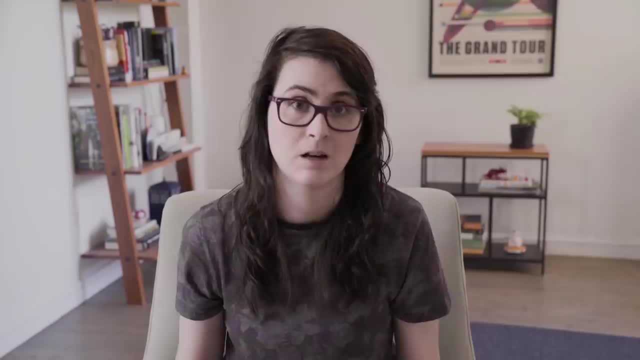 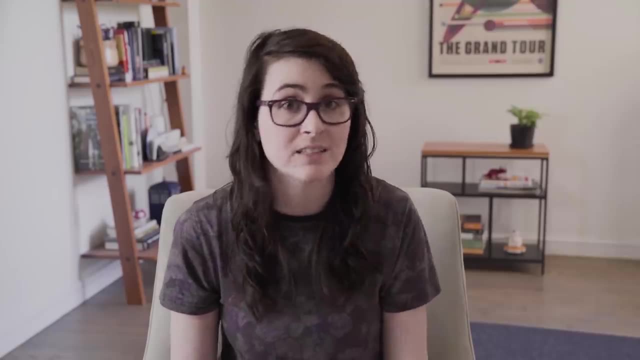 we're gonna feel it. Correction, we already are. But who is we here? In theory, climate change is a global problem. The average global temperature is increasing, But who feels the effects of that temperature increase and all the ramifications from heat waves to hurricanes to flooding That isn't evenly distributed? 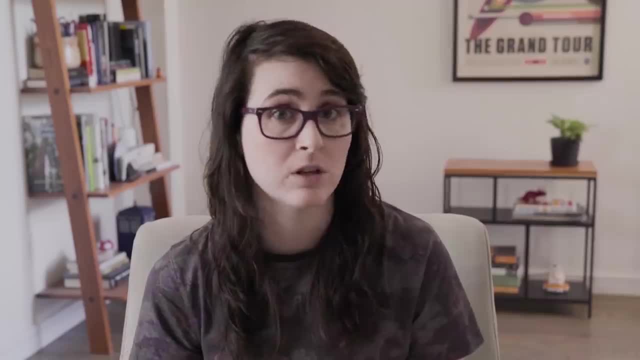 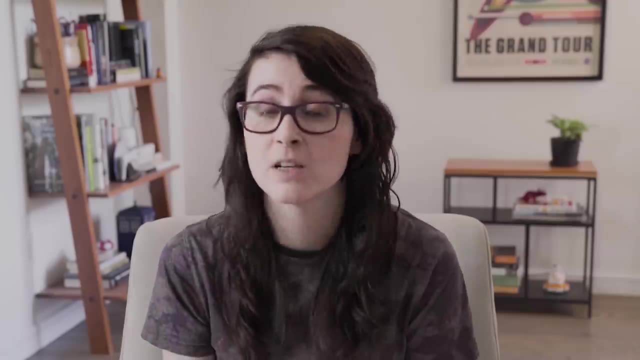 Disproportionately. the impacts of climate change fall on low-income communities and communities of color. Wealthier and often whiter communities with more access to resources can in some ways buy themselves out of the worst impacts. This inequality is called environmental injustice or climate injustice, And if you want to learn more, we've made a whole playlist for you. 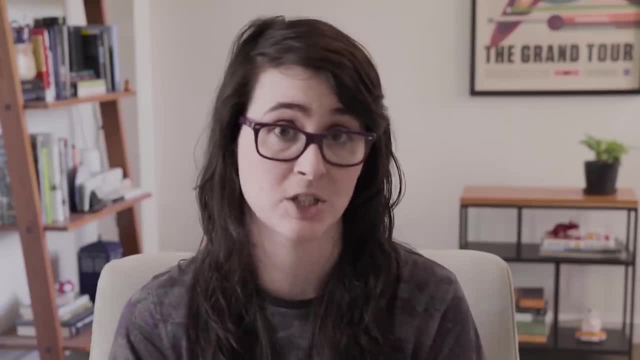 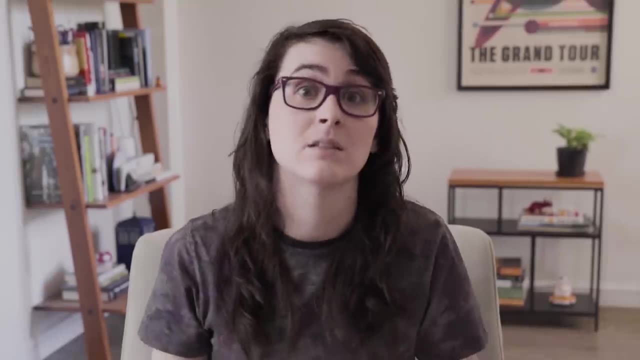 to watch. So what's to be done? That's the big question when it comes to climate change And unfortunately, there isn't a single answer. The global climate is a massive, interconnected system, So we need big solutions And we need solutions for everyone. 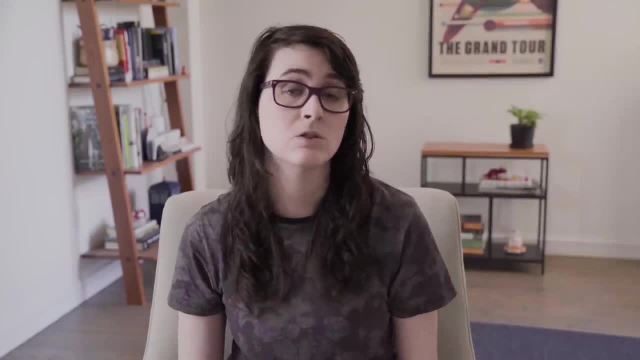 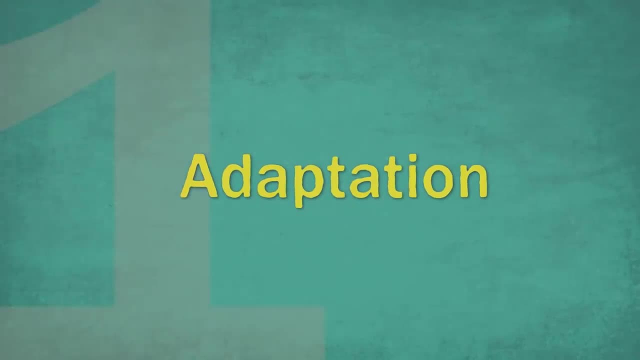 not just the folks with the biggest paychecks. Generally speaking, though, these solutions fall into two categories: adaptation and mitigation. We can adapt systems and structures to the new and future climate systems In response to sea level rise. this means building flood barriers. 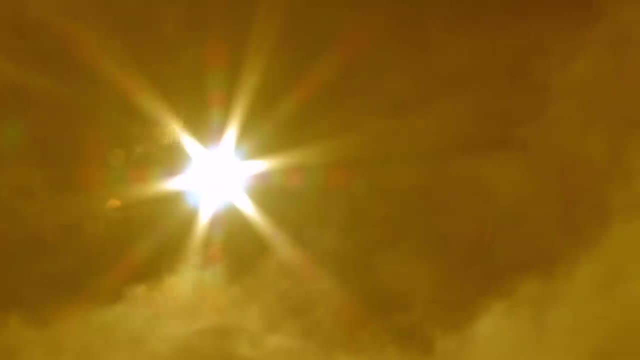 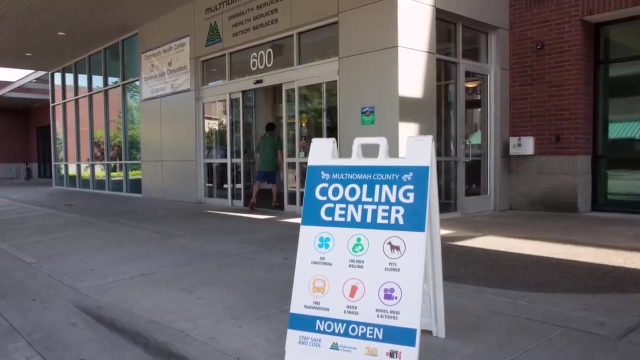 removing homes and businesses away from low-lying coastal areas As temperatures rise. adaptive measures look like drought-tolerant crops or cooling centers, which are free, air-conditioned spaces for people to escape deadly heat. Adaptation also means developing policy and governance structures to support people displaced by sea level rise or cyclones. 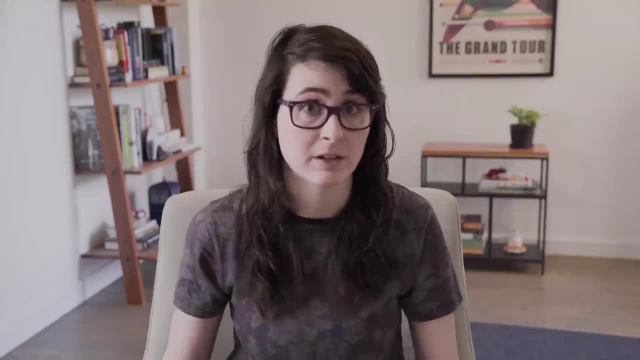 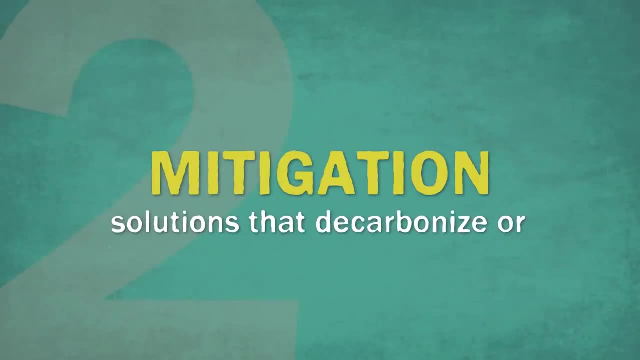 or droughts. Adaptation helps preserve human life and systems by responding to the impacts of climate change, but it doesn't tackle the cause of climate change. emissions Mitigation strategies are solutions that decarbonize or reduce greenhouse gas emissions, like replacing coal and gas power plants with renewable power generation.